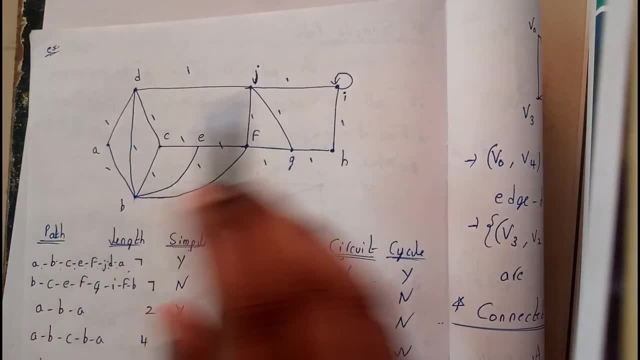 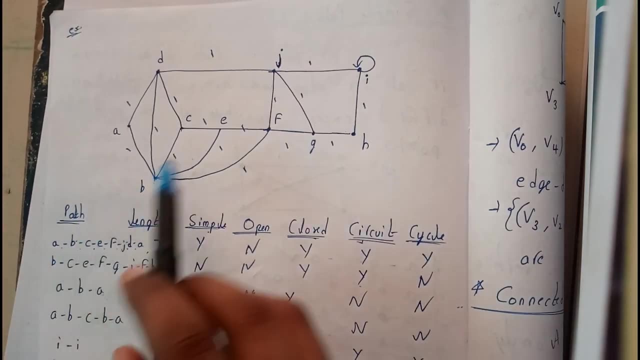 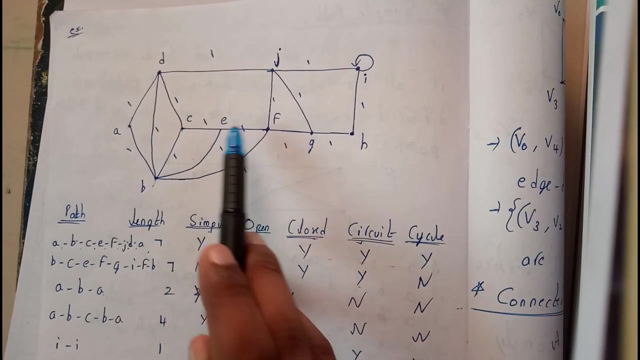 with an example. So here is a graph with every edge labeled with a weightage of 1.. Okay, so let us take the path A to B, sorry, A to B, B to C, C to E, E to F, F to J, J. 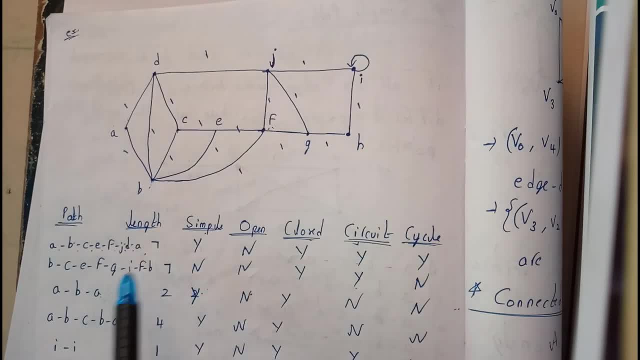 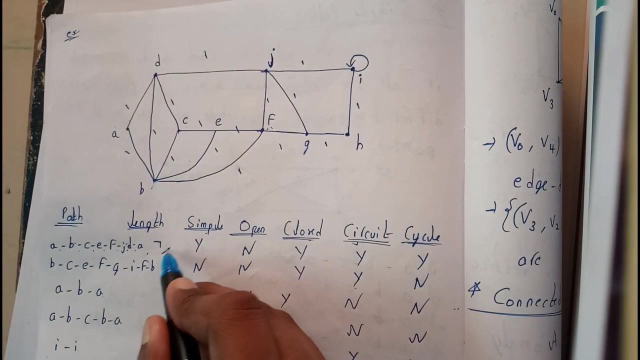 to D, D to A. I think we have traveled all the paths 7, A to B, 1.. 1,, 2,, 3,, 4,, 5,, 6, 7.. So the length is 7.. Okay, are there any parallel edges or some? 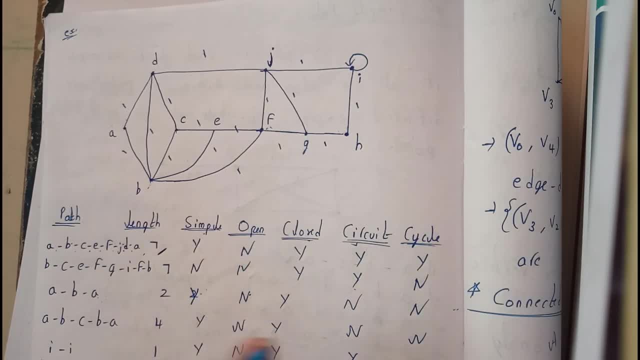 kind of self loops. There are no parallel edges and no self loops. So this is a simple graph. Is it an open graph? What is an open graph? Open graph: it has initial and final positions. should be initial and final vertices should be different. 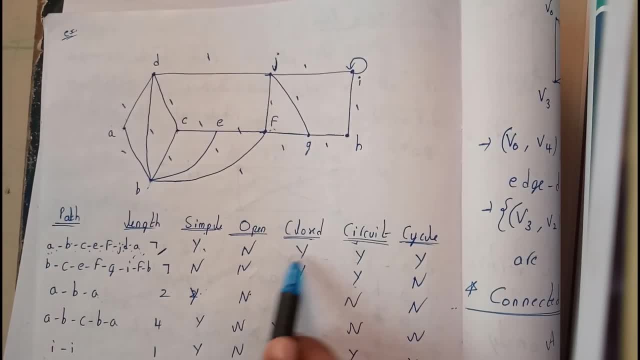 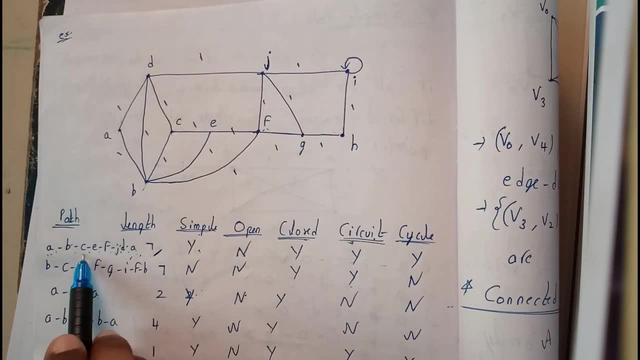 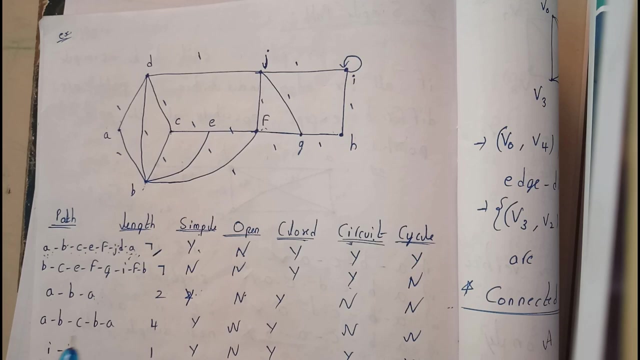 Whereas here they are same. So this is a closed, not an open. So when we will be checking for a circuit, a circuit will be having no repeated may have repeated. it should not have any repeated edge. Here there is any repeated edge. No, I think there is no repeated. 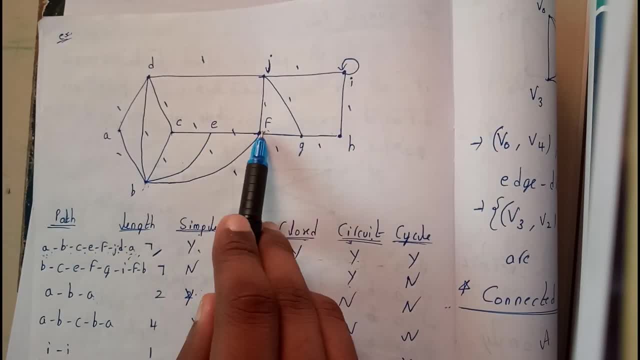 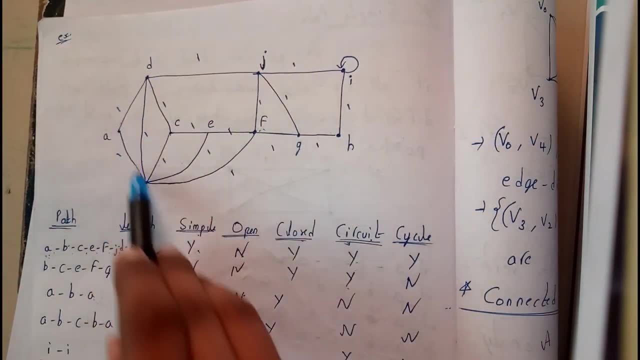 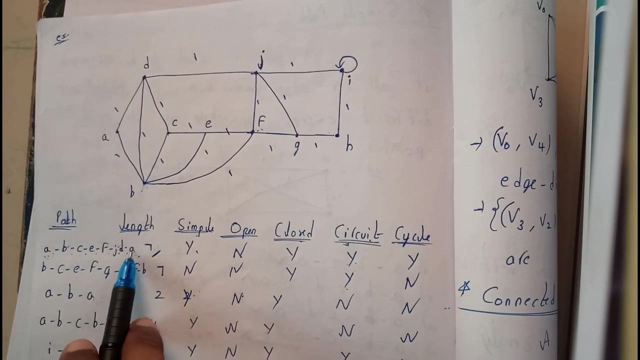 edge. if we have traveled like this- C to E, E to F, F to J, J to D- There is no repeated edge. We have just rotated like this. So there is no repeated edge and no similar vertex other than the both. So this is a cycle. Every cycle is a circuit. 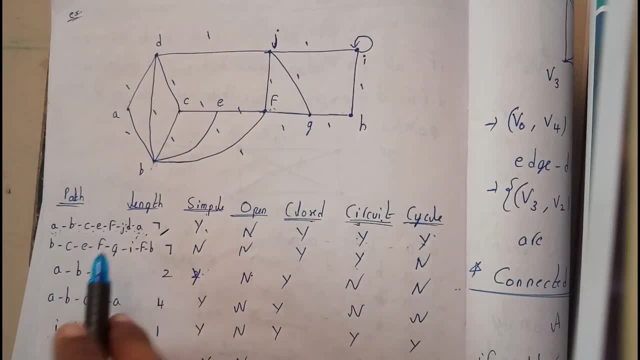 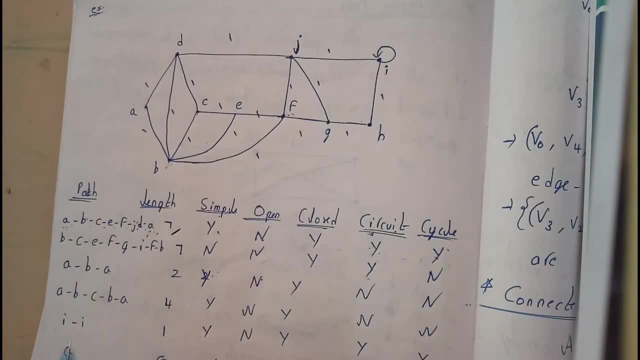 So, yes and yes. So let us take the next example. I will be going two examples and you try to solve the rest of the examples. I think I have written around 5 to 6.. Okay, let us take the second example. 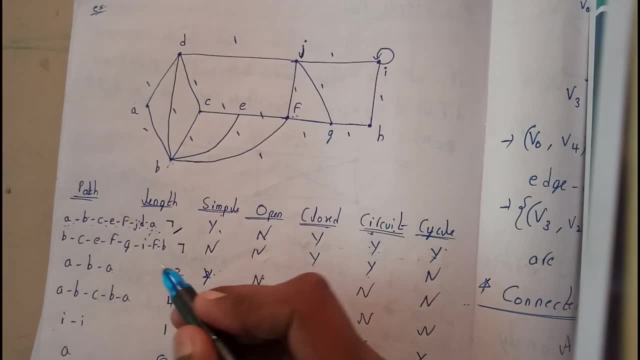 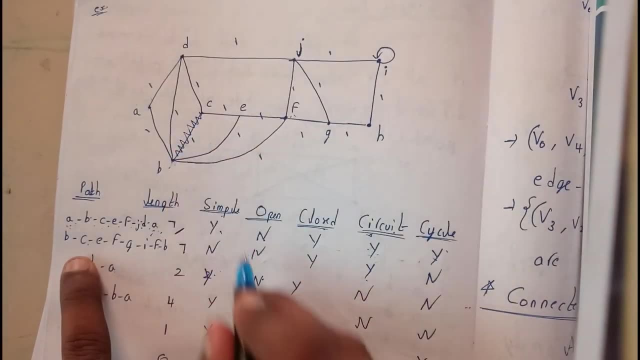 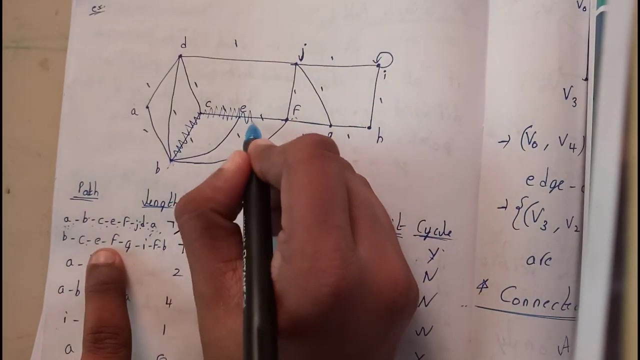 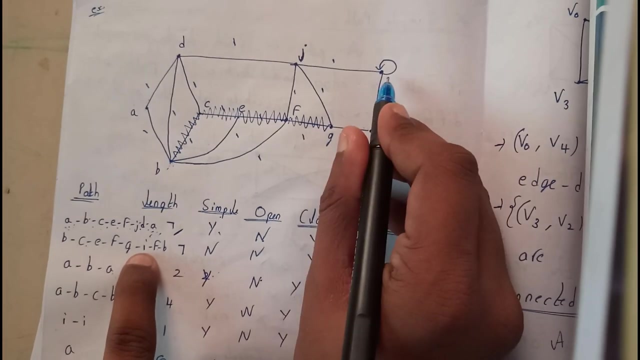 Okay, let us take a pen. We will be drawing so that it will be clear. So: B to C- okay, B to C. C to E- okay, E to F. F to G, G to I- sorry, G to J, I think so, okay, G to J. 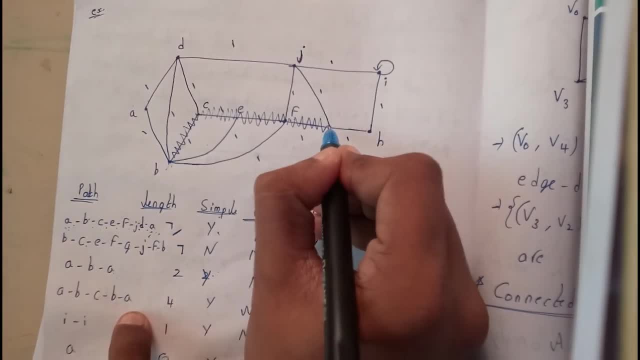 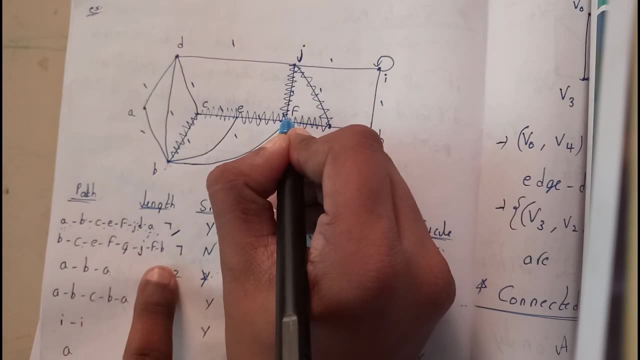 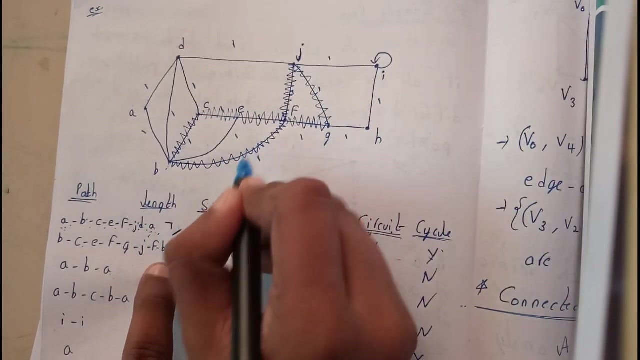 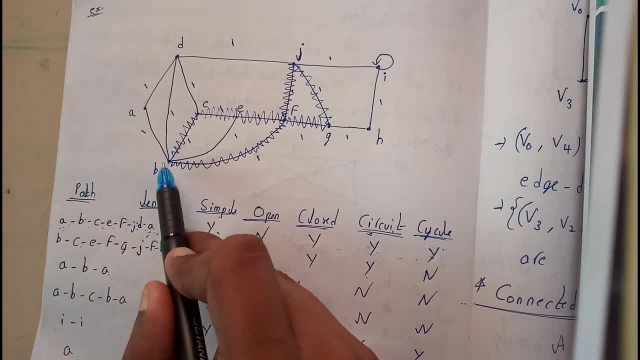 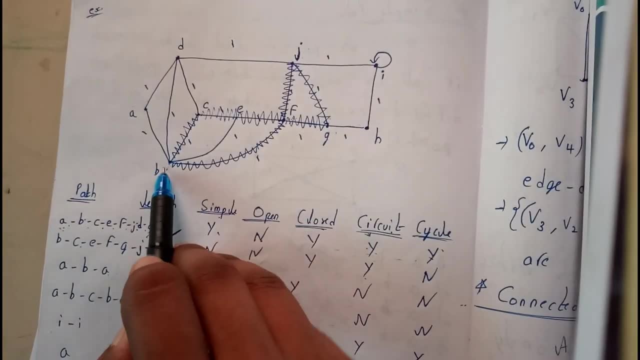 I think this explanation, this kind of explanation, was better. We have travelled B to C, C to E, E to F, F to G, G to J, J to F and F to B. So the initial and final positions are: 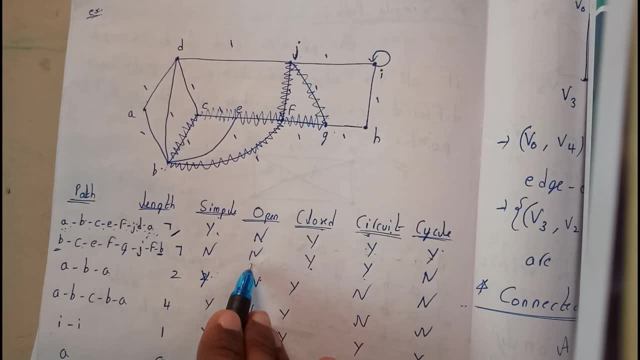 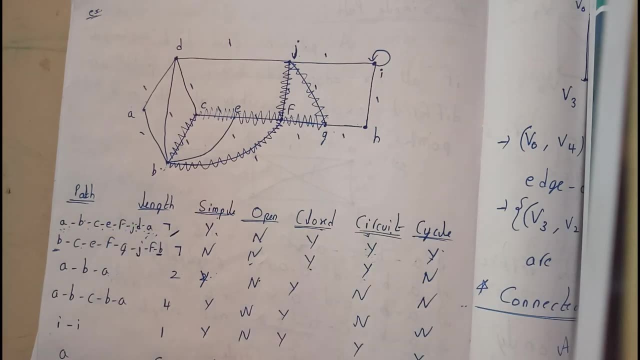 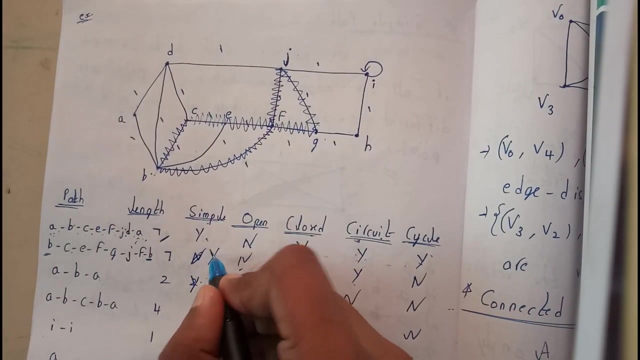 same. So hence it is a closed And we will be open for the. let us write no. And are there any parallel edges? Yes, there is a parallel edge. Sorry, there are no parallel edges. So this is a simple graph. Okay, This is a simple graph, And the length of 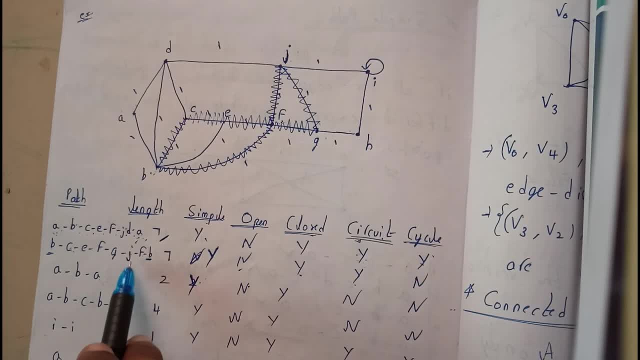 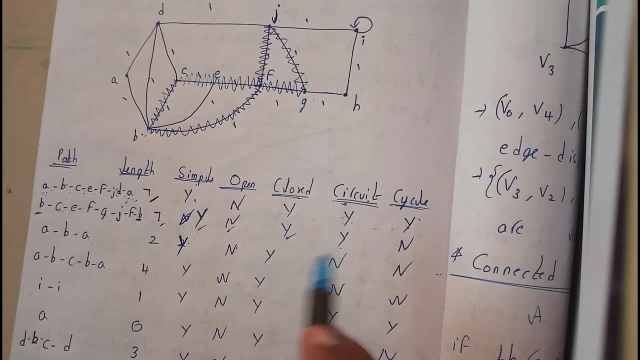 length 1,, 2,, 3,, 4,, 5,, 6,, 7.. Length is 7. And it is a simple graph And it is a closed, not an open one. And whenever we will be going through circuit, Okay, Circuit initial and 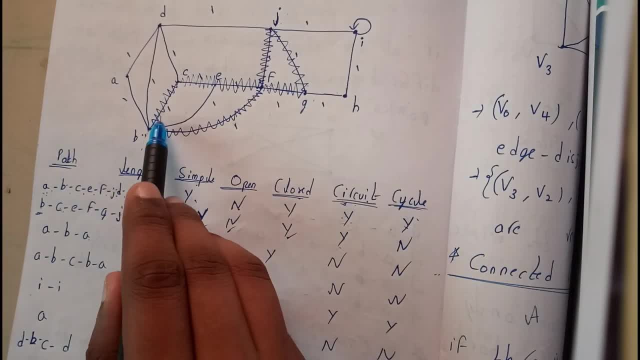 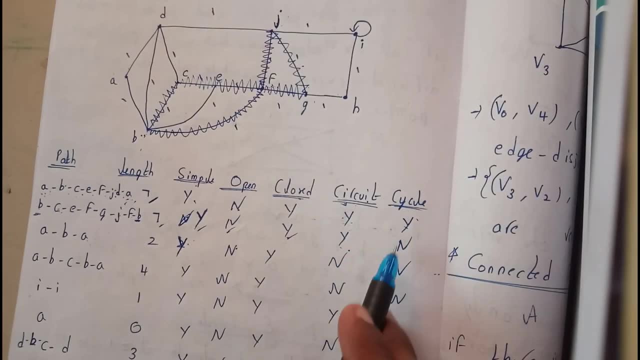 final positions are same. We did not pass through the same edge twice. We have passed once, once, once, once, once, once once. So it is a circuit. Whenever we will be coming through cycle. there is a repeated vertex. We have visited on B. 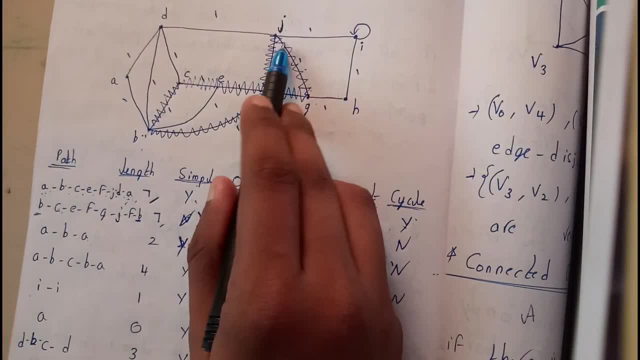 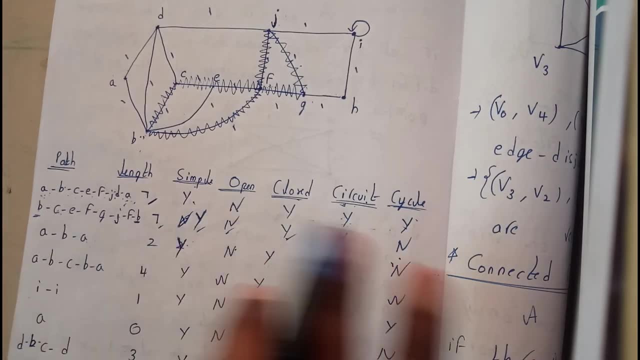 Both the paths. Initially, I traveled like this: I visited this once And I visited it again, So this is not a cycle. That's it. I think everyone is clear with all the concepts up to now. Thank you for watching. If there are any doubts, down you will be finding comment.